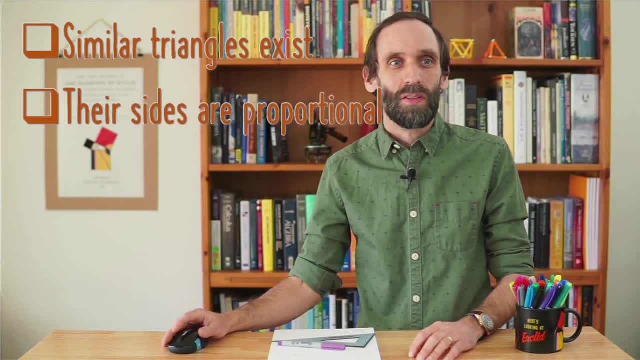 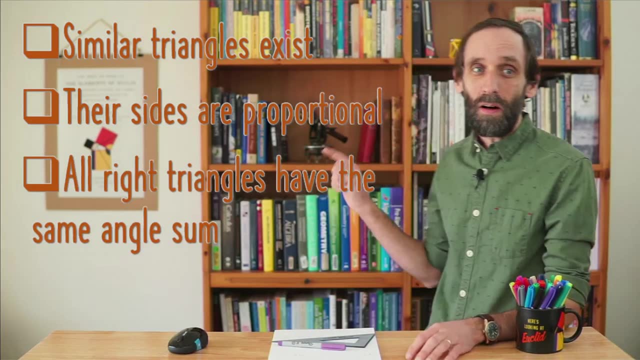 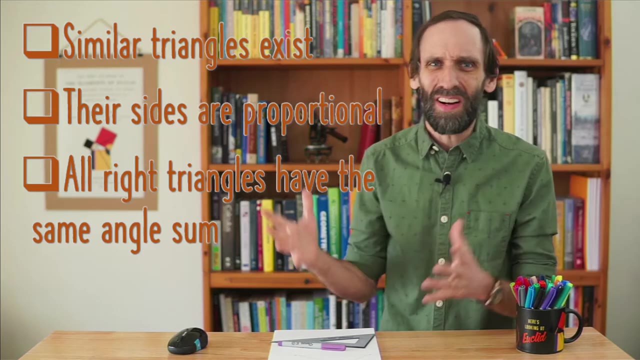 exist. We assumed that. oops, we've assumed that the sides, the corresponding sides of similar triangles are proportional. and we've also assumed that, all right, triangles have the same angle sum. and maybe you're starting to think: wait a second, aren't we going to verify? 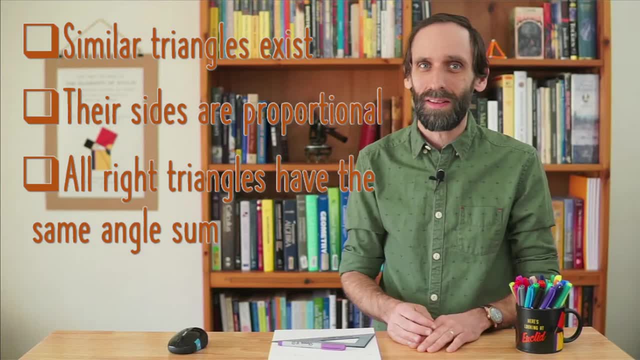 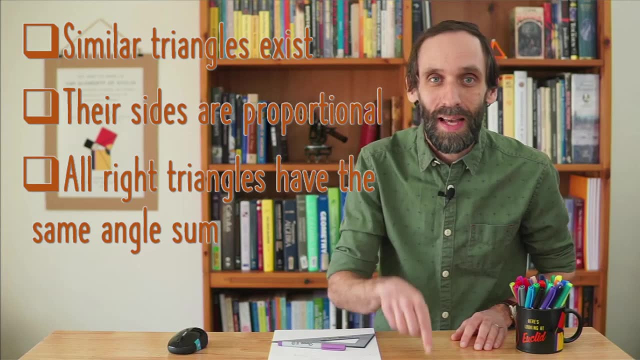 it. Is there anything in this unit? Is this just all assuming things? And you know, what is all this built on? Well, I've got good news for you. If that's what you're thinking, in this lesson we 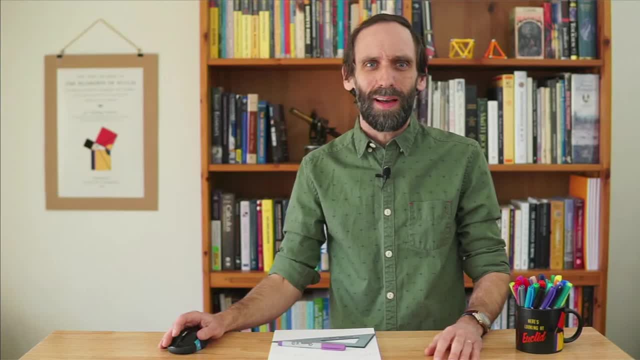 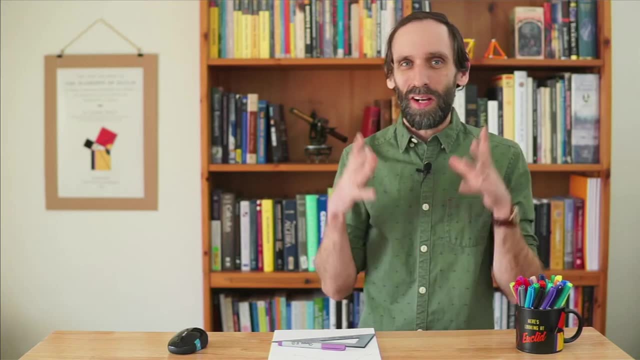 are going to do our first proof. okay. Now, maybe that's bad news for you. Maybe you're like: oh, no proofs, that's scary, I don't like proofs. but you know, I'll try to make it as clear and 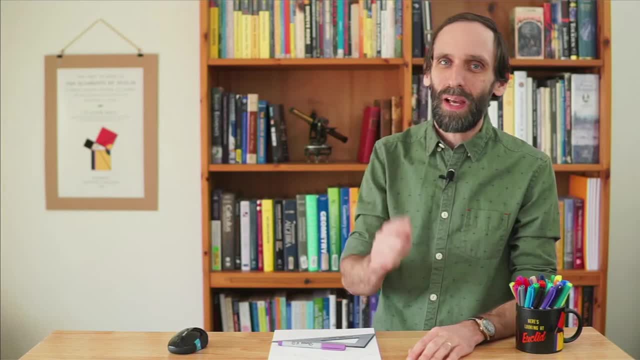 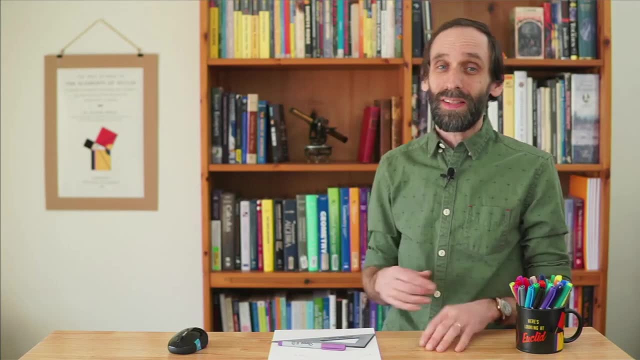 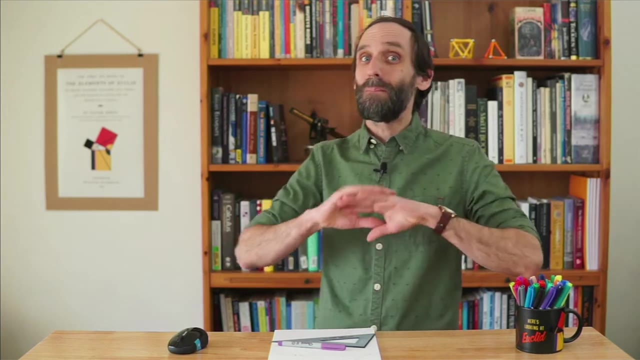 comprehensible for you as possible, but I cannot pass up the opportunity to do this proof for you. in this lesson We're going to prove the Pythagorean theorem. Mathematicians seem to think that this proof thing is really important, so also, let's appease them, shall we Now keep in mind there are many. 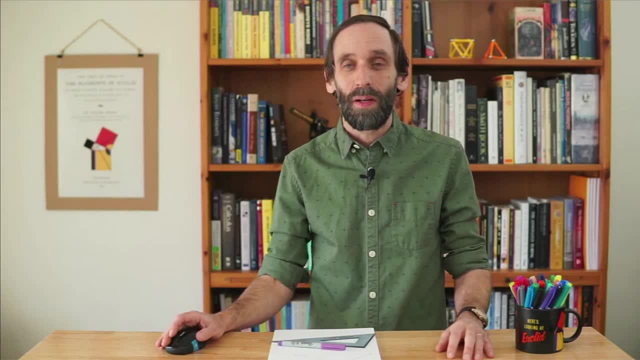 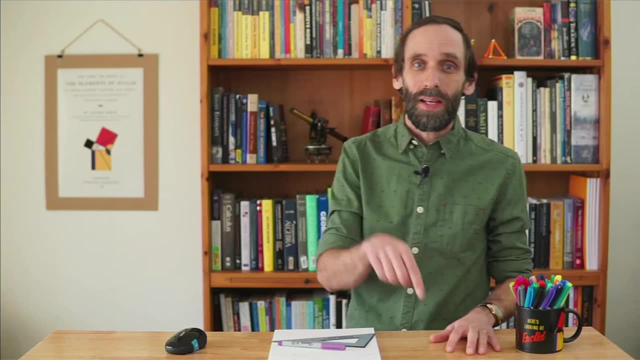 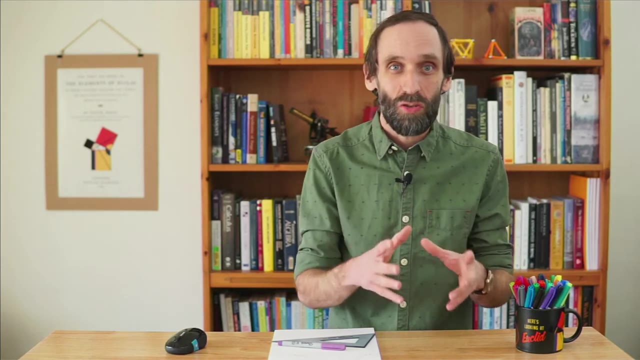 many proofs for this Pythagorean theorem. Actually, this picture on the wall is a diagram for one of those proofs, not the one that we're going to be doing today. Today, we are going to do a lovely proof, in my opinion, which is based on this idea of similar triangles: The fact that 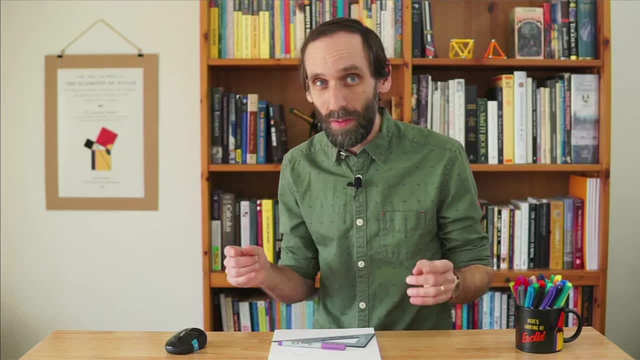 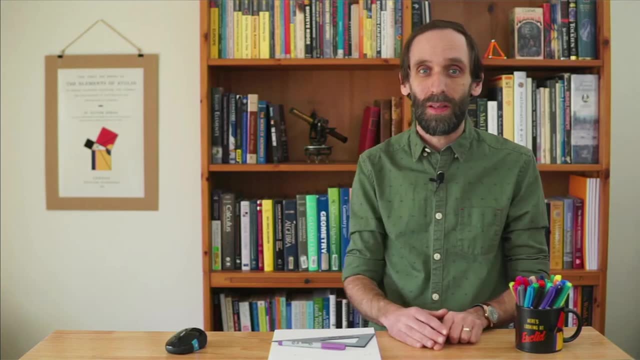 similar triangles have corresponding sides that are proportional. that's what this proof is based on, and it's something we've been talking about a lot, so I thought this would be a great point in the course to do this proof. Now, as I've mentioned already, Pythagorean theorem super. 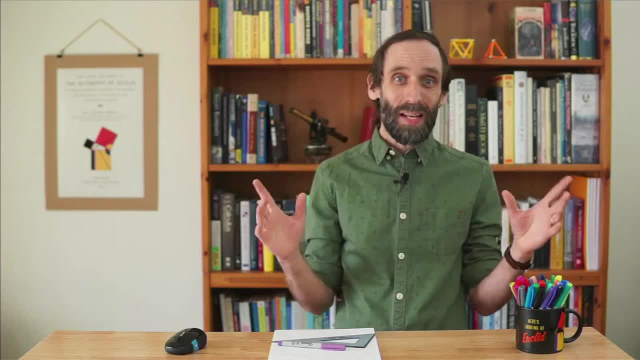 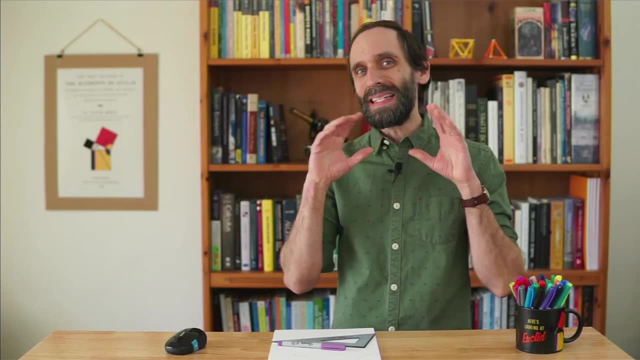 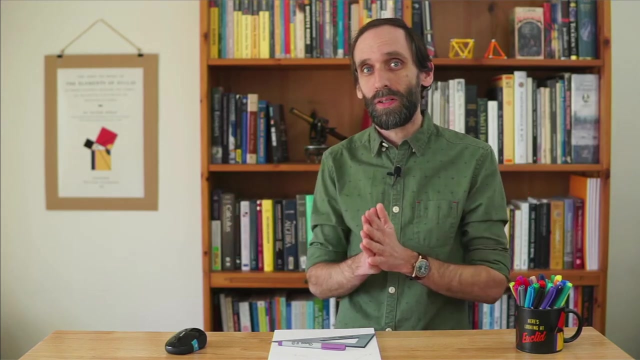 famous, probably the most famous theorem in all of geometry, possibly in all of mathematics. but a couple things to keep in mind about the Pythagorean theorem is, even though it is named after Pythagoras, the Greek mathematician Pythagoras is known well before his time. okay, So Pythagoras did not invent or discover the. 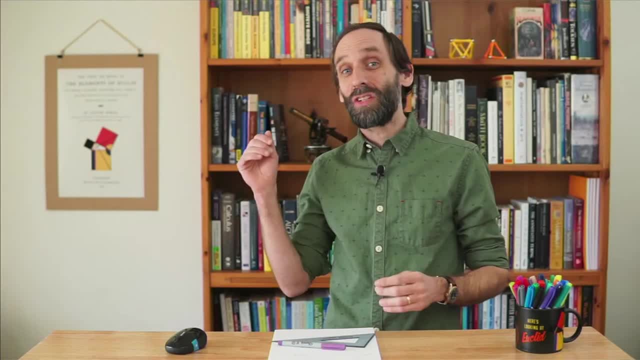 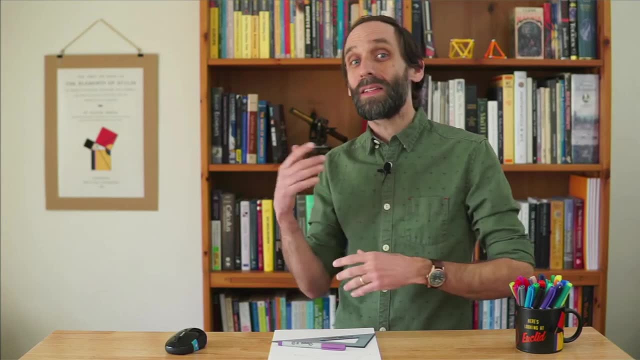 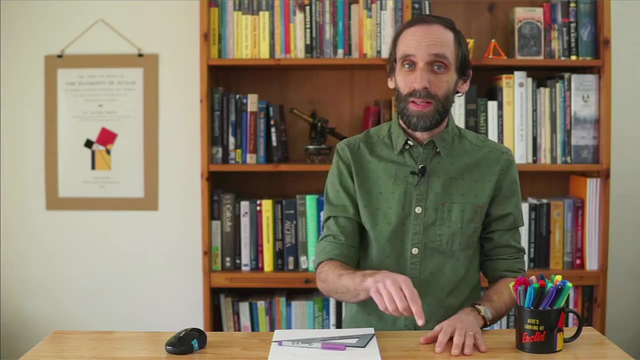 Pythagorean theorem. In fact, evidence indicates that ancient Indian, Egyptian and Babylonian mathematicians used and were familiar with at least some form of the Pythagorean theorem long before Pythagoras. Now, this will not be the last time we discuss this theorem I'm bringing 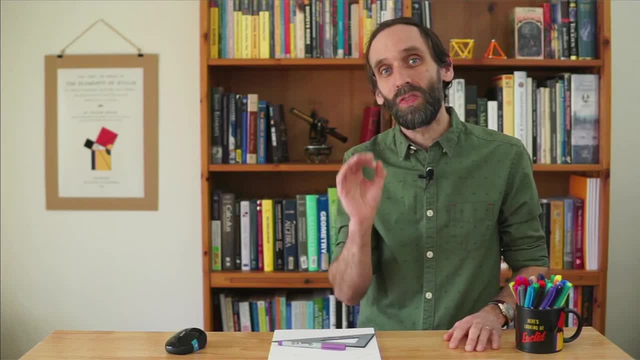 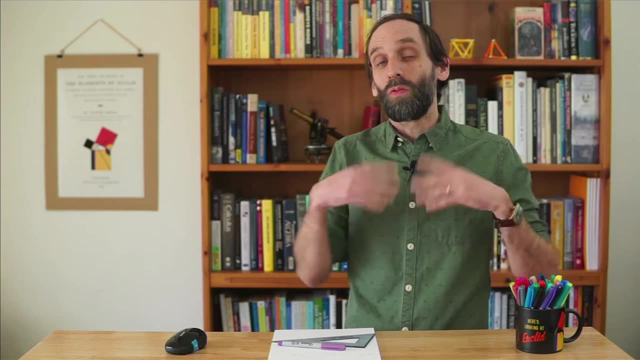 it up right now in this unit because it's a very useful tool For measurement. okay, this is a unit all about measurement and right now we're talking about right triangle, trigonometry, right Measuring, right triangles, and you can use the Pythagorean. 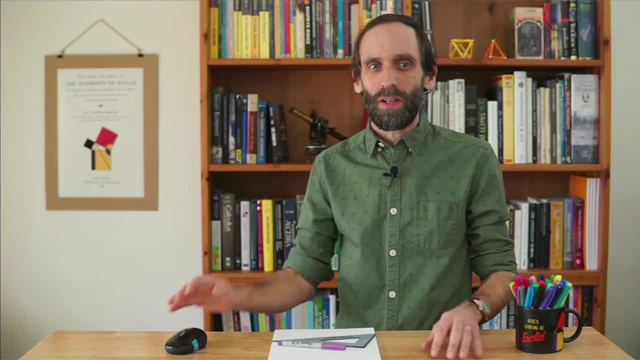 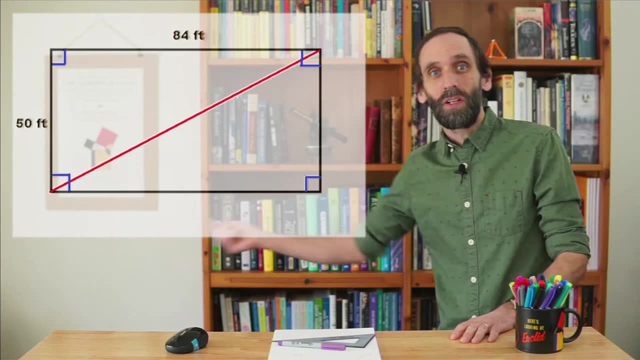 theorem to measure right triangles. So it's part of right triangle trigonometry. So a couple things you can measure with the Pythagorean theorem. Let's say you have a rectangle and you know the height of the rectangle. you know the length, the width, whatever the height, the base. 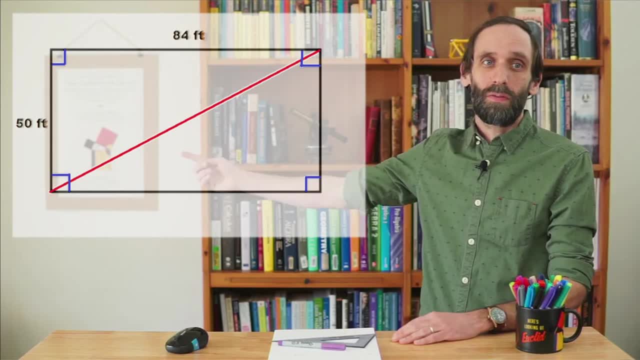 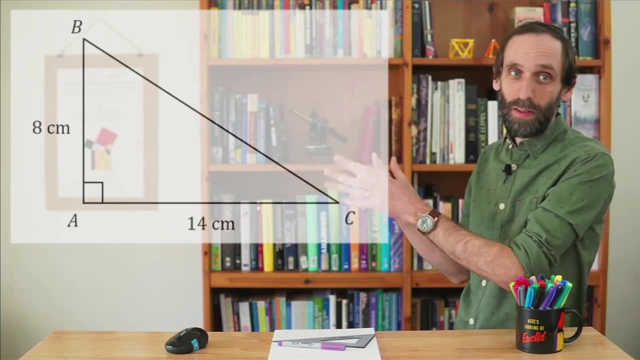 You can use those and find the diagonal of the rectangle, what you see here in red. That's one use. and then another use is that if you have a right triangle like this one, if you know any two sides of the right triangle, you can. 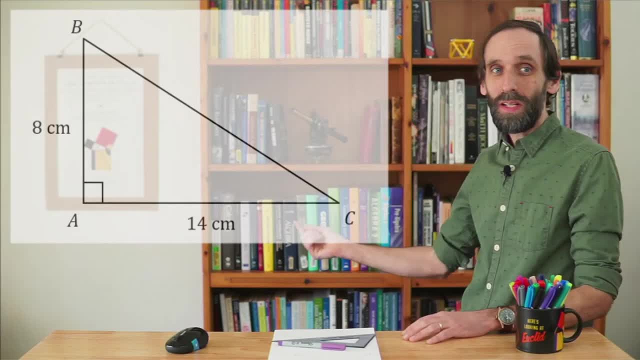 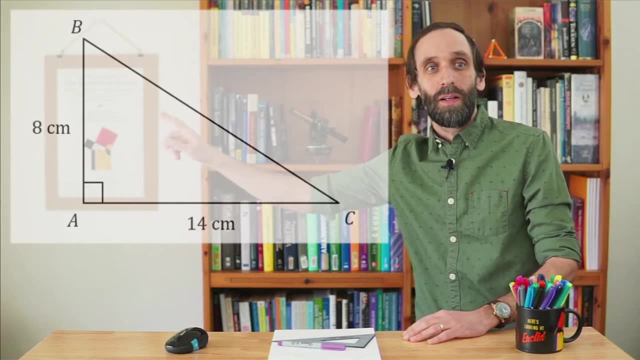 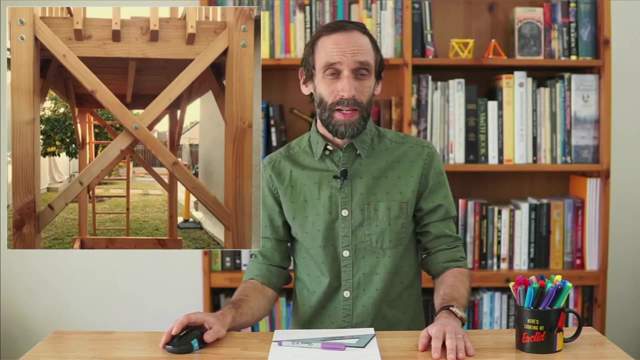 find the third side with the Pythagorean theorem. So you see, here the base is given and the height is given, but the hypotenuse is not given. So, given the base and the height, you can find the length of the hypotenuse using the Pythagorean theorem. So in case you, oh yeah, 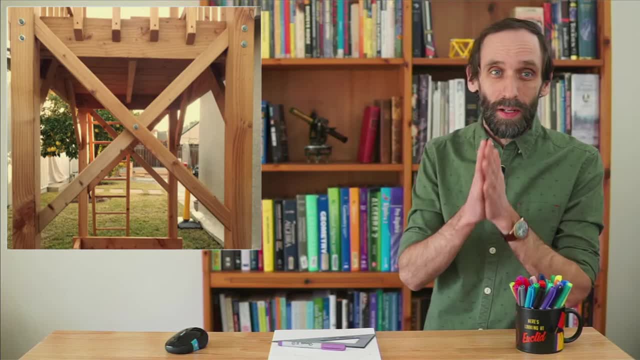 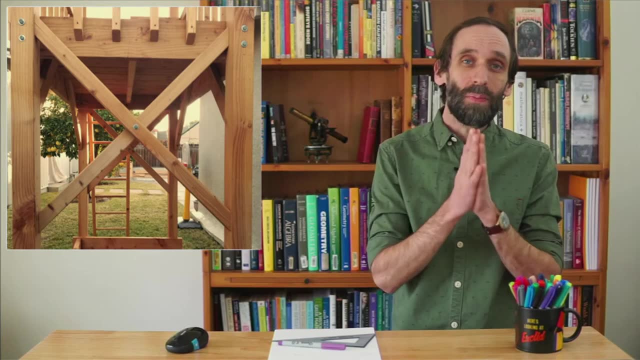 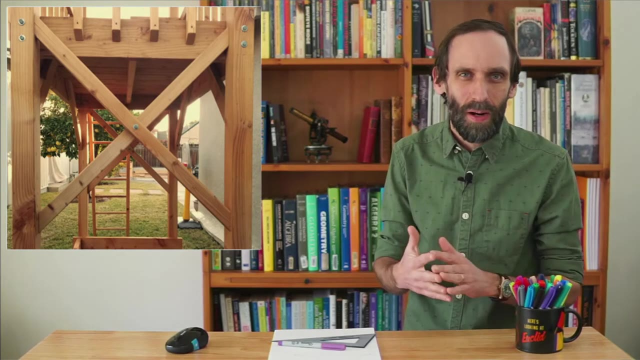 I was going to mention this In the last unit. we used trig ratios right sine cosine tangent to find the length of those cross beams. We could use the Pythagorean theorem instead. So we'll look at that later in the unit how we could use the Pythagorean theorem instead of sort of the two-step. 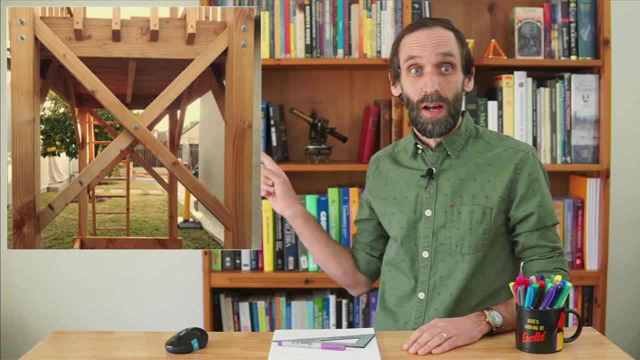 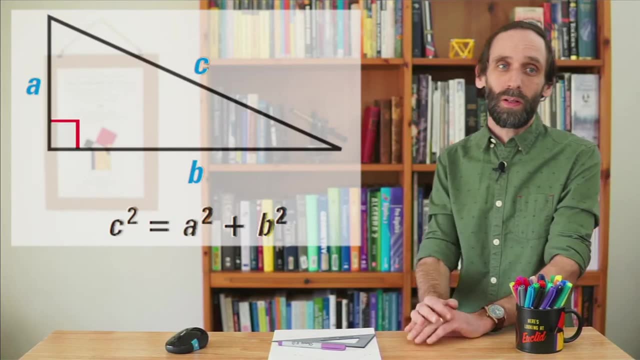 process, using the trig ratios to solve a problem like this. Now, what is the Pythagorean theorem? In case you don't know, I'll give you the statement of it really quickly here. Now you know, people might say: oh yeah, I know the Pythagorean theorem. It's a squared plus b squared equals c. 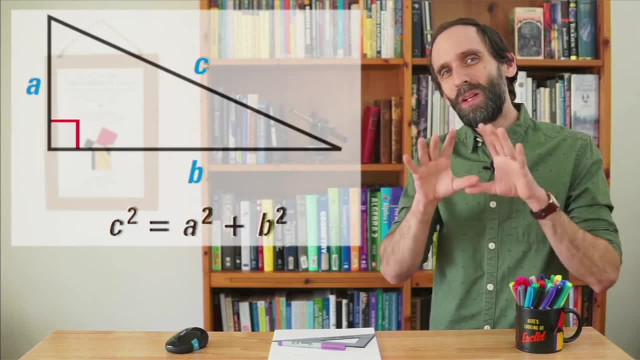 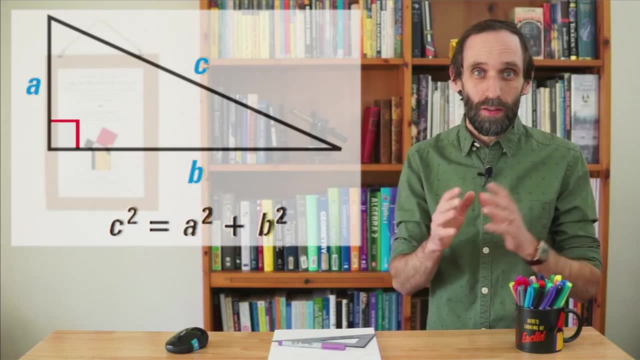 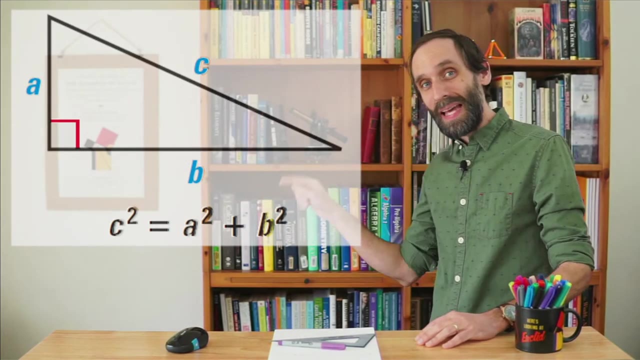 squared. Well, yeah, that's true, but it's important to set it up properly. Okay, so in order to use the Pythagorean theorem, you need to start with a right triangle. So, given a right triangle with length, side lengths a, b and c, where a and b are the legs, the shorter side and c. 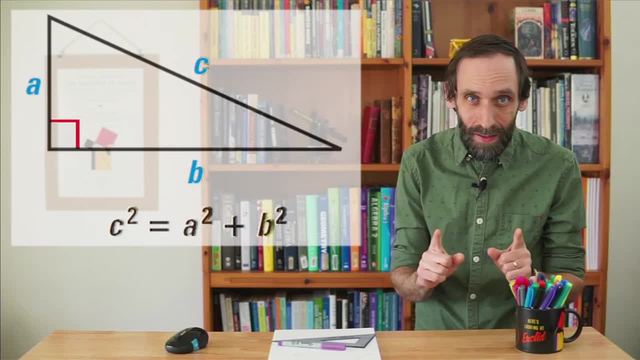 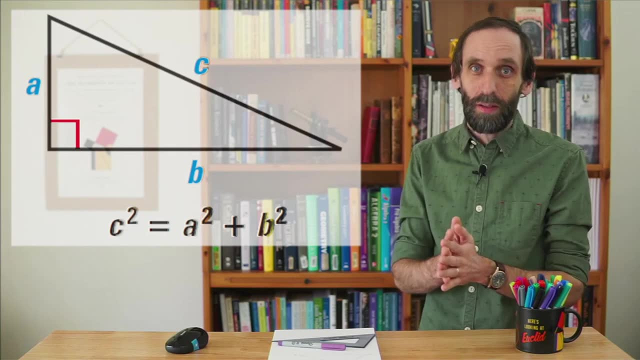 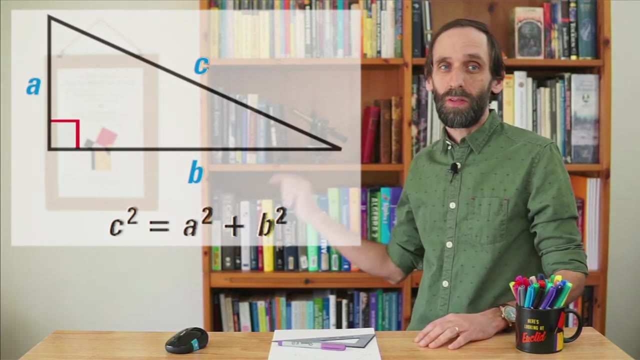 is the hypotenuse, the long side. then a squared plus b squared, equals c squared. Okay, so you have to set it up properly. You have to have a right triangle and the two shorter sides are a and b and the longer side is c. In that situation, a squared plus b squared equals c. 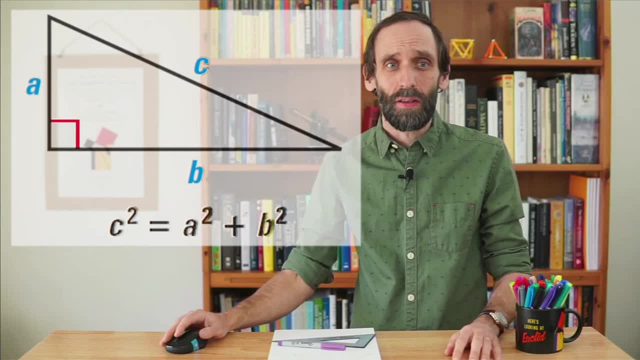 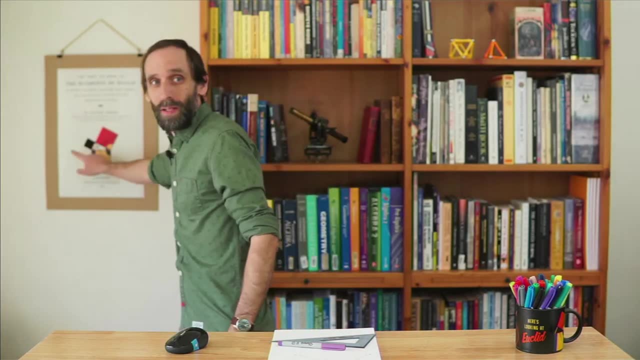 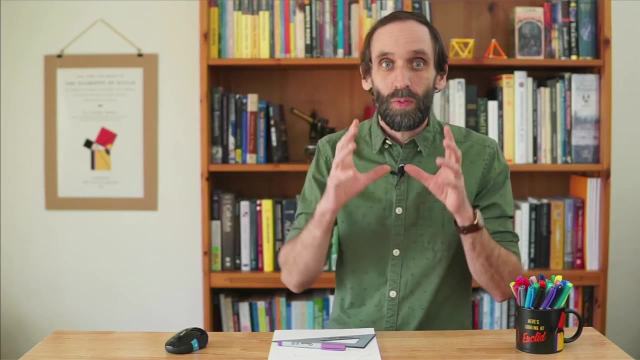 squared. Now, when the Greeks did this, they actually thought of these as real squares, which is one reason I like this diagram. by the way You know, it shows that this square plus this square is equal to that square, The physical square areas. when you add them up, you know the squares of. 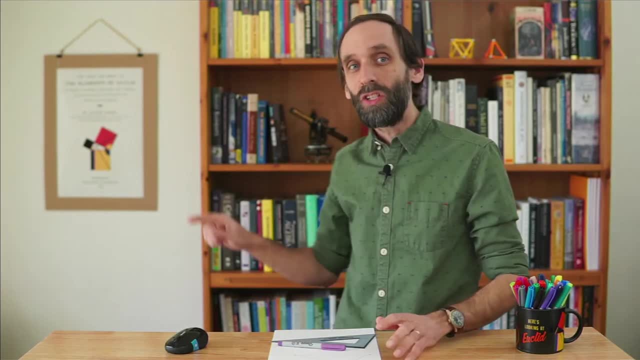 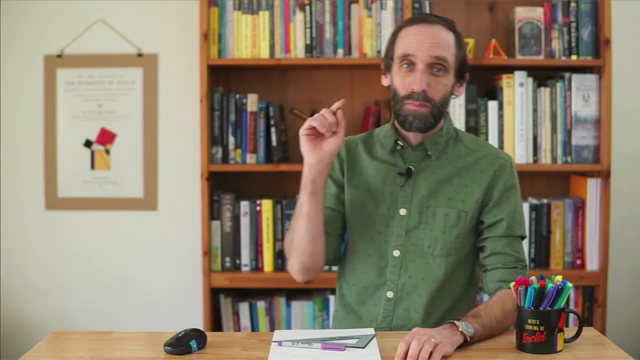 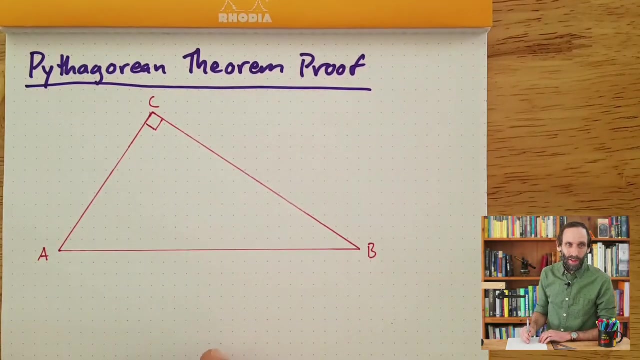 the shorter sides. when you add those two areas up, you get the square of the long side. Okay, so that's enough setup. I think Let's dive into our proof for the Pythagorean theorem using similar triangles. Okay, so the first thing we need before we prove the Pythagorean theorem is we need a. 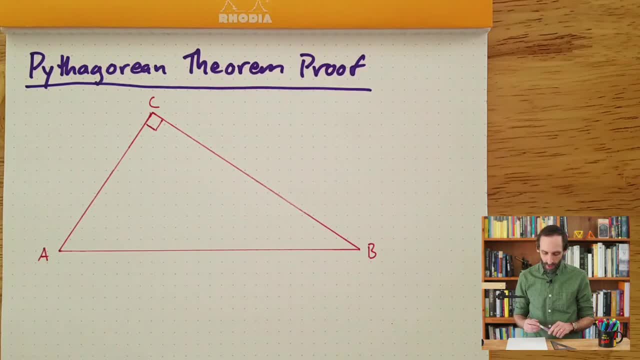 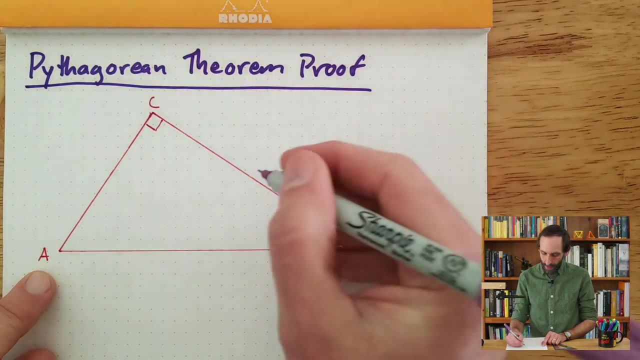 right triangle. So here you see, on my paper, I have a right triangle with points labeled a, b, c. Let's label these sides as well. Now the convention is to label the side across from the angle with that lowercase at that point. So this is angle a, point a, and so this will be side a. 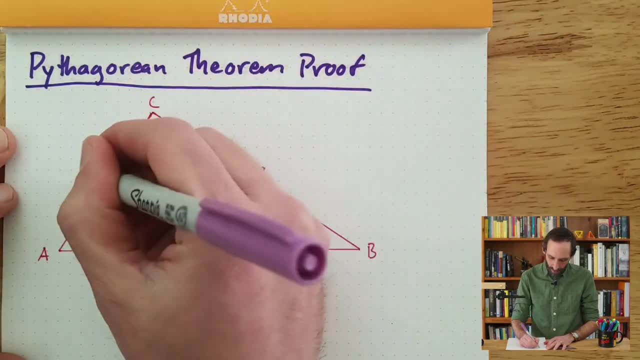 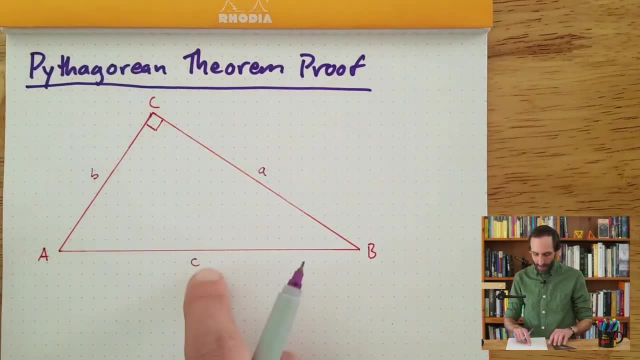 and then b will be over here, across from b, So this side is b and then down here c. I mean with a c it kind of looks like the uppercase c, but that is a lowercase c Now, keep in mind. 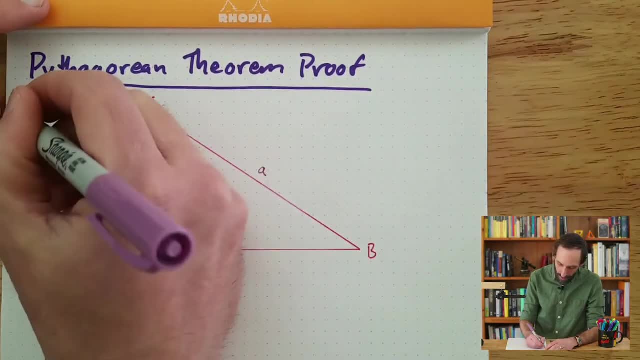 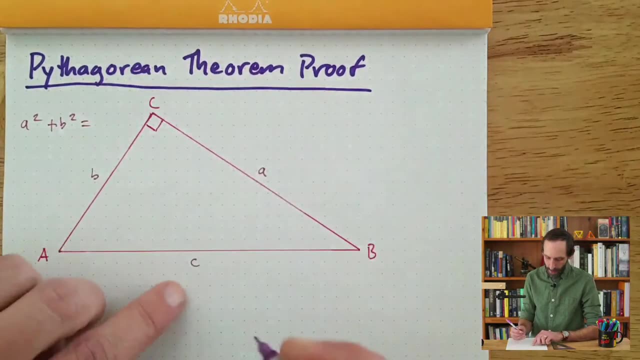 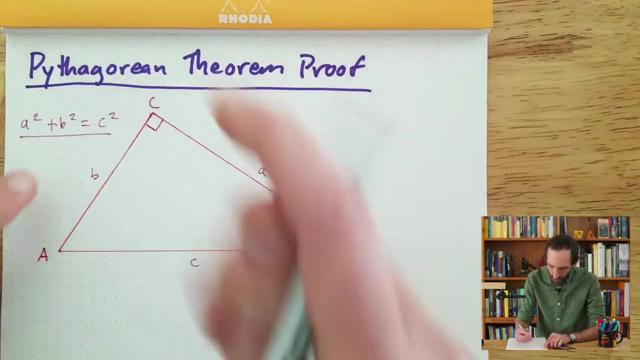 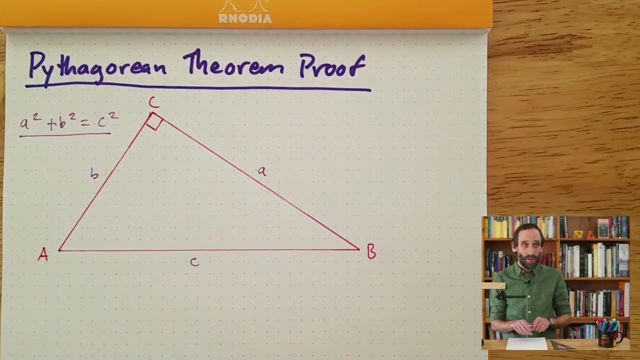 the thing that we're trying to prove is that a squared plus b squared is equal to c squared. Okay, this is our goal: to prove that the squares of these two shorter sides, when added together, is equal to the square of this longer side. Now, the first step in this proof: 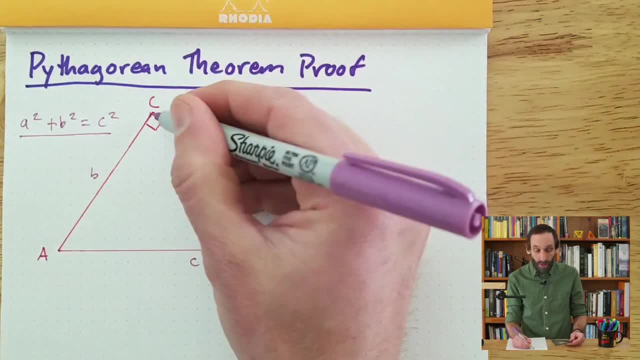 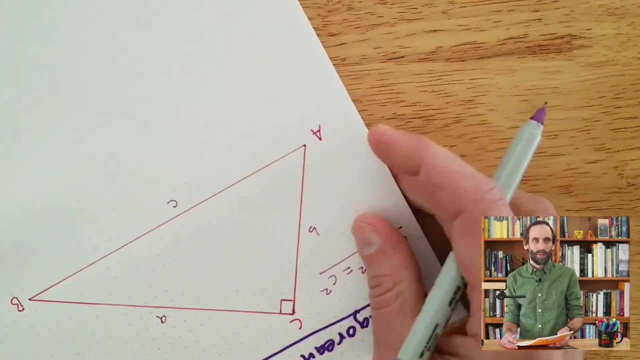 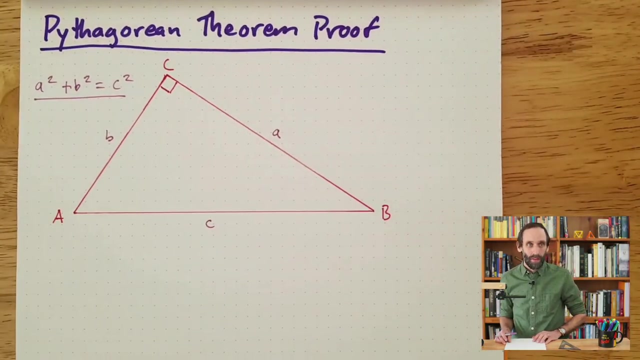 is to drop a perpendicular from the right angle down to the hypotenuse. Now you know, oftentimes you'll you might be used to seeing right triangles oriented this way or this way. For this proof, it's easier to have that right angle at the top. I think it makes it a little bit easier. So we put. 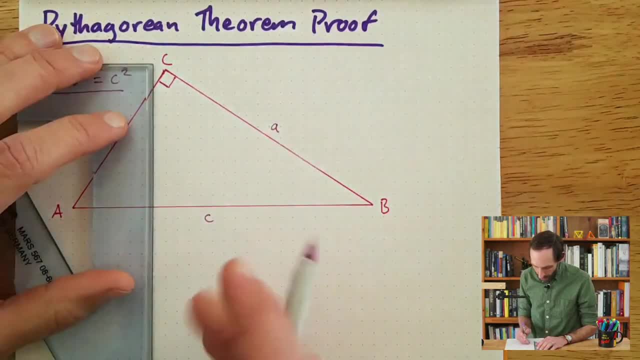 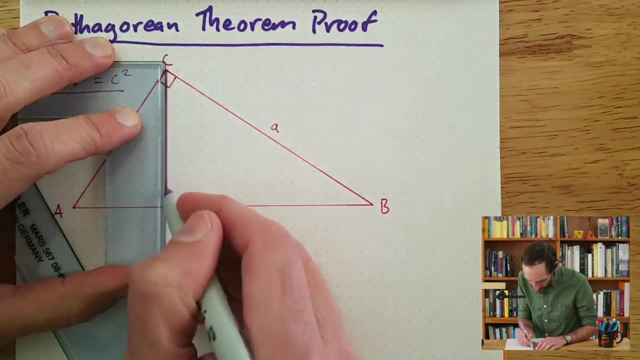 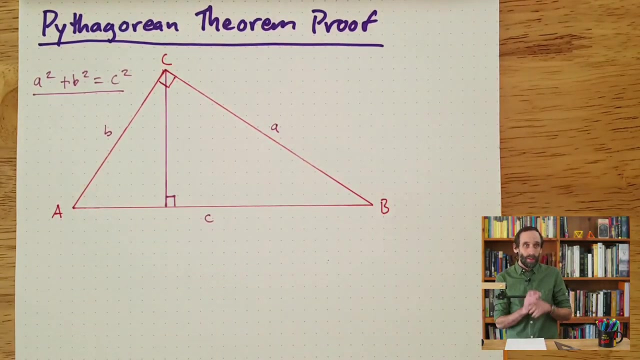 the right angle at the top and we drop a perpendicular from the right angle down to the hypotenuse, And so let's go ahead and do that. I'll use the dots of my dot grid paper to get that perpendicular in and I will specify: there is my right angle. Now I'm going to need to label a few. 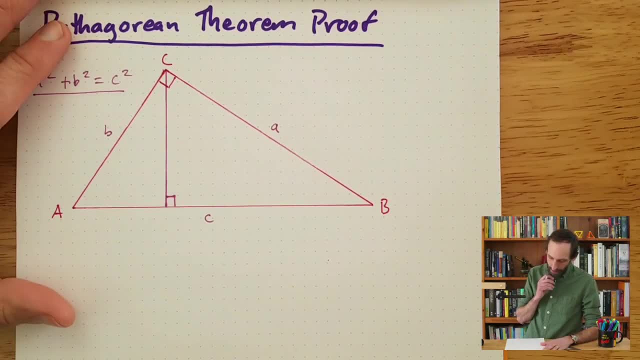 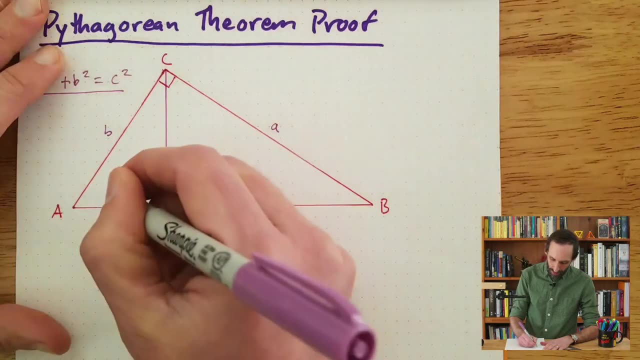 things. Okay, let's start by labeling two lengths here. Now you see this length right here. it's part of length c, but it's not the whole thing, so I want to give it its own variable. I'm going to call that x And you see this. 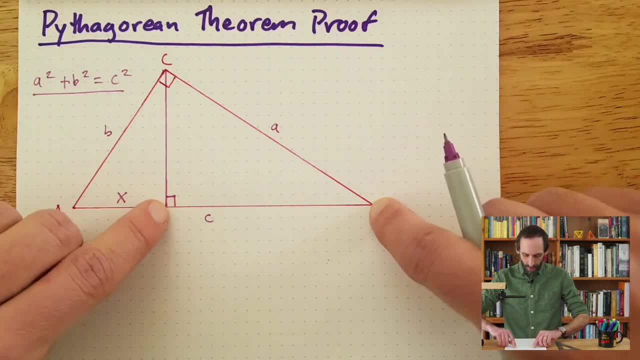 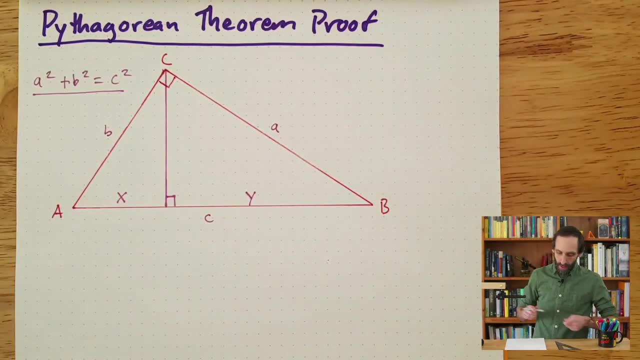 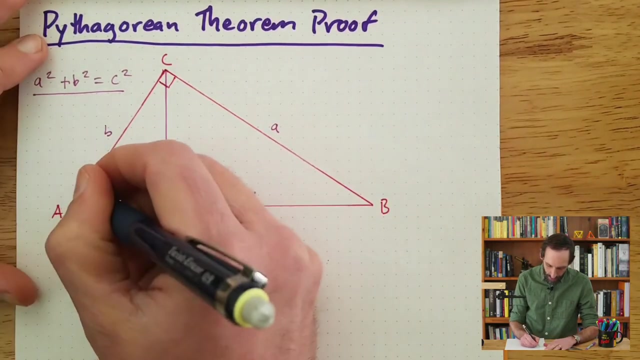 length right here, also part of C, but again not the whole thing. so I'm going to label that length Y. We'll give our own variables there. Now I also want to label a few angles. Okay, I'm going to do this with a pencil and you'll see why later. This angle down here. 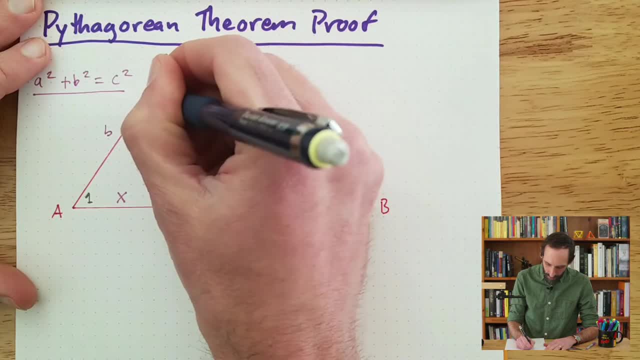 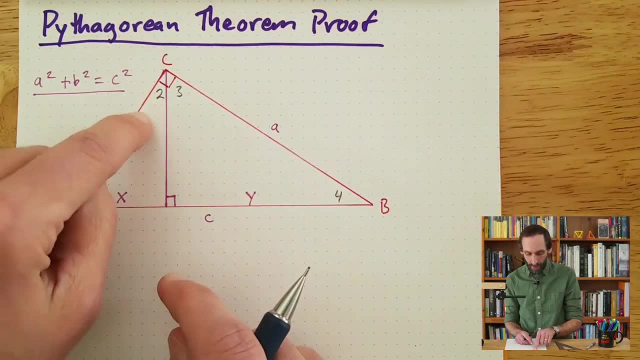 I'm going to label this as angle 1, then this one will be 2, this one will be 3,, this will be 4.. Now, keep in mind, the 2 is part of a right angle, but it's just this part, and 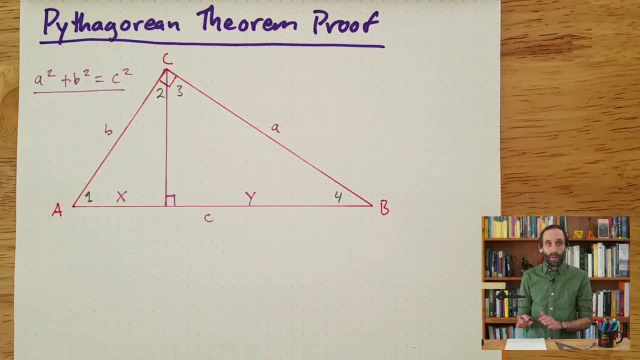 the 3, also just that part of the right angle. Now, before I can, you know, use this fact about proportionality of similar triangles, I need to prove, or at least give you some argument for, why there are similar triangles in this diagram. Okay, and the thing that 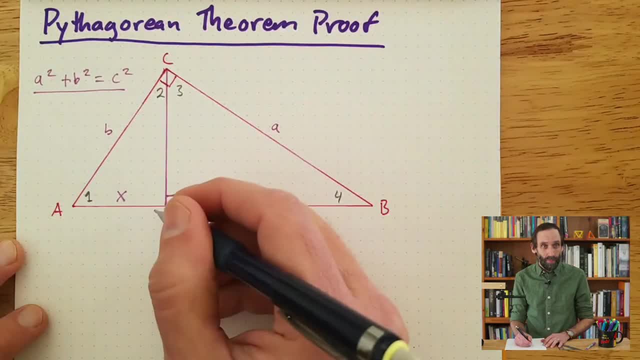 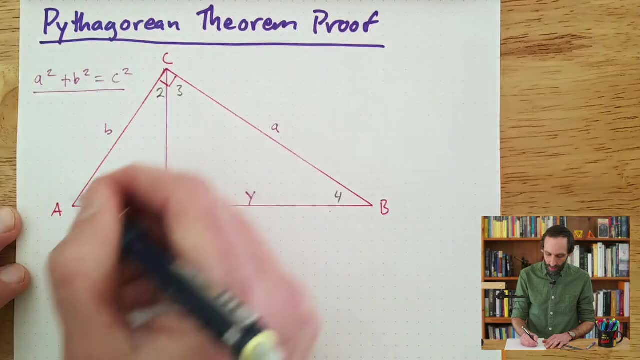 I want to show you is this small triangle right here is similar to this sort of medium size triangle. Okay, so this small triangle right here is similar to this sort of medium size triangle, and both of those are also similar to this large triangle. So before 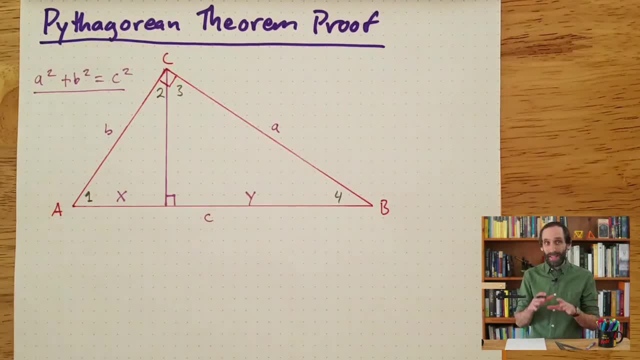 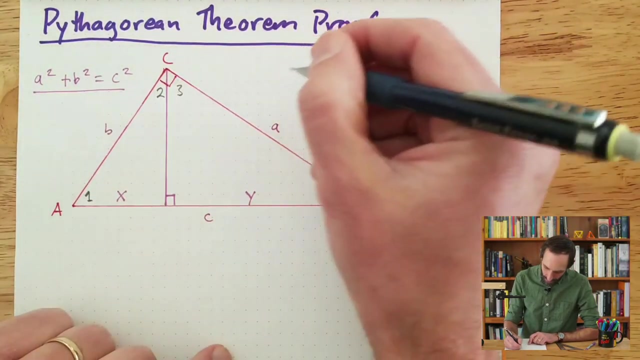 I need to. before I can do the proof, I need to demonstrate that that is actually true. This is how I'll do it. I'll use the fact, the assumption that we've been making that all right triangles have the same angle sum. So I'll start with a small triangle and I'll 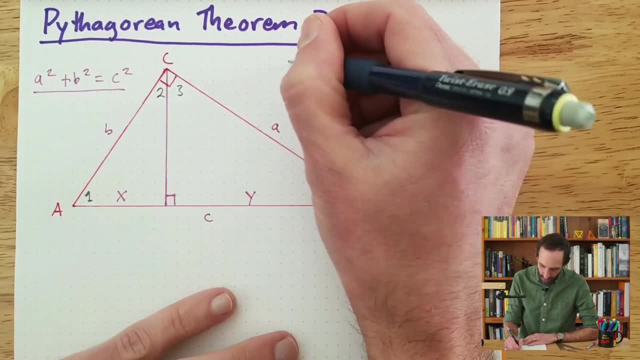 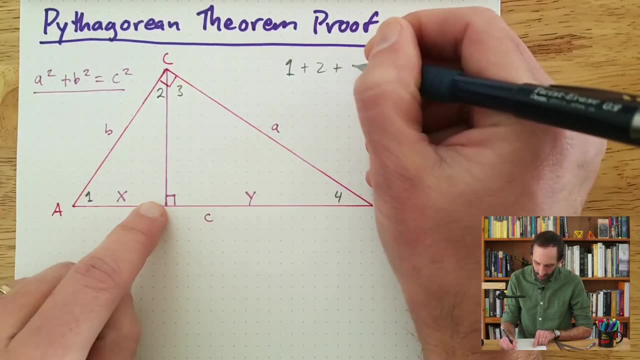 say: well, wait a second. what's the angle sum of the small triangle? Well, it's going to be 1. Plus 2 plus 90 degrees. This is a right angle here. Well, that is equal to the angle sum of the big right triangle. And let's see that one is 1, plus 4, plus well, it's both. 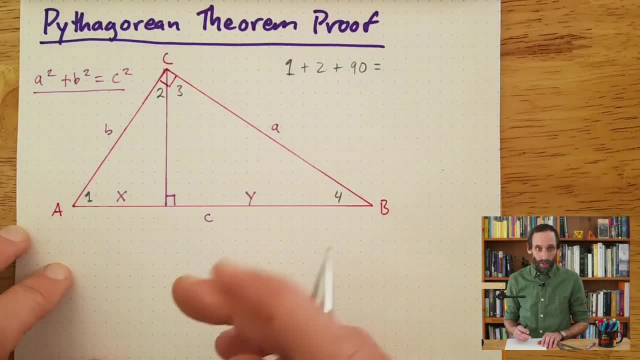 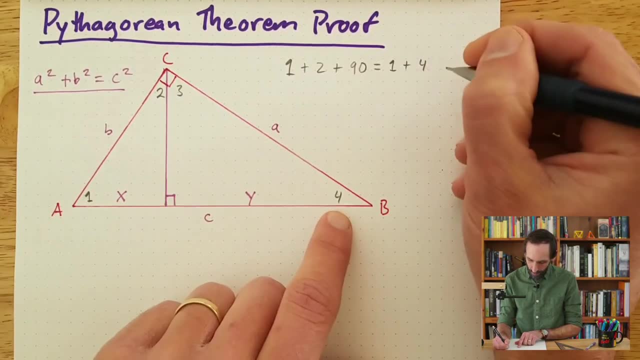 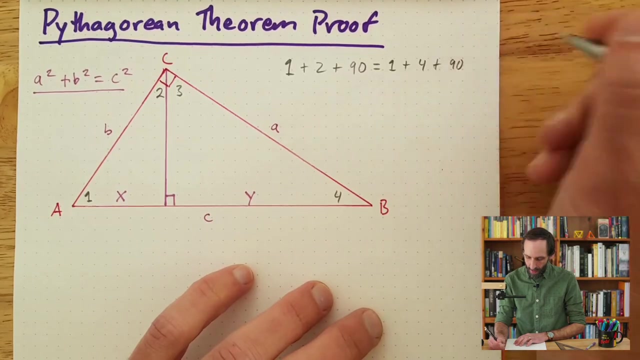 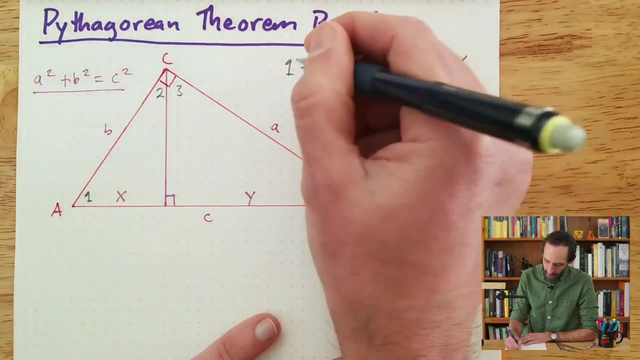 of these together, so it's 90 degrees. So plus 90 degrees. Okay, now what I want to do is cross these out. I can also cross these out, and I see that 2 is equal to 4.. So let's. 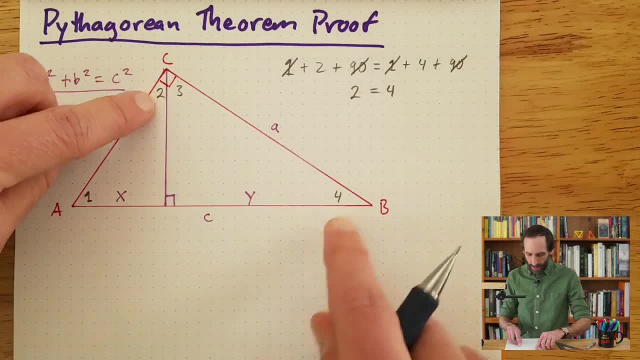 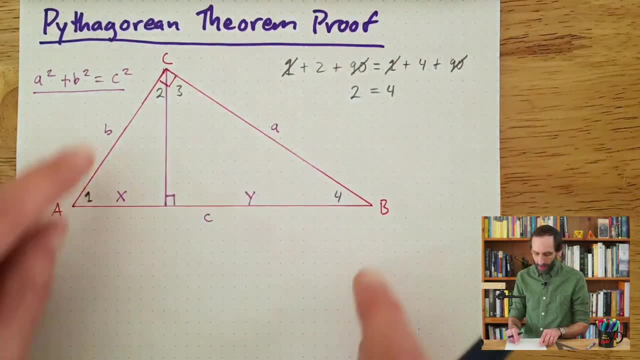 write that 2 is equal to 4.. So that means this angle and this angle are equal. Now I can do something similar. I can do something similar to show that angle 1 is equal to angle 3.. Let's use this triangle. 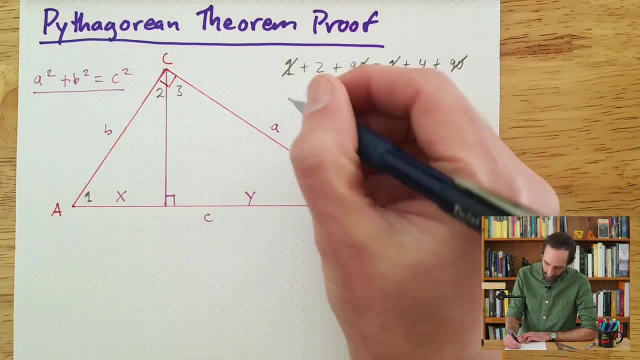 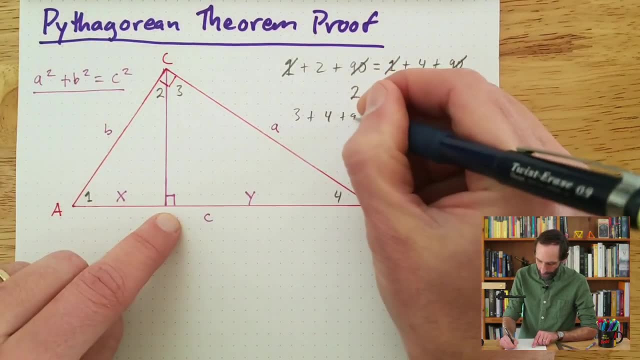 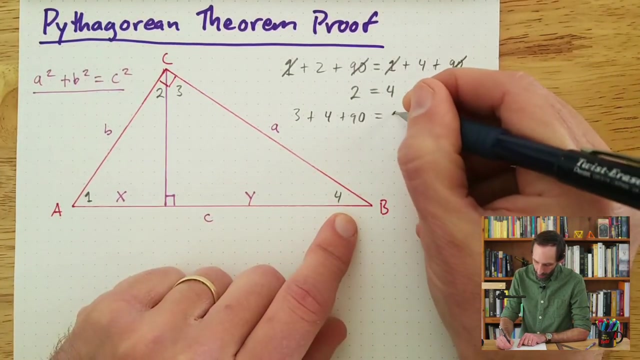 over here. So I will write down here that angle 3 plus angle 4, this one plus this, one plus 90, is equal to using the big triangle, angle 1 plus angle 4.. So 1 plus 4, plus again the 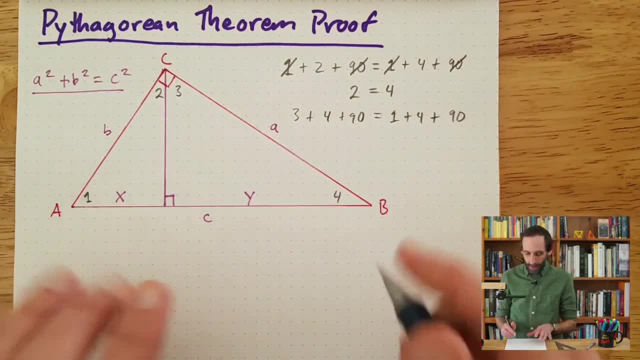 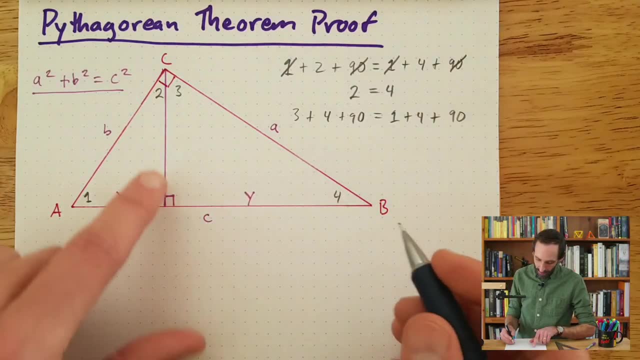 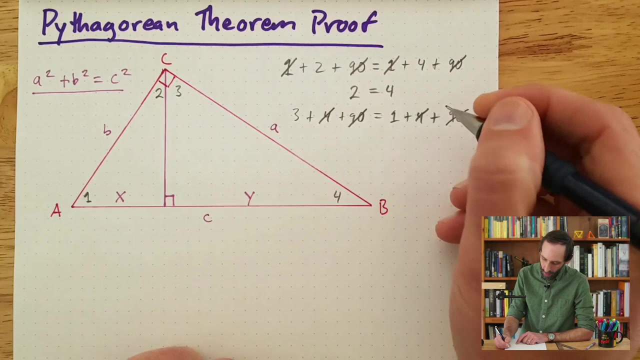 90 degree angle up there, And I'm setting these equal using the fact that, using the assumption that all right triangles have the same angle, sum is what enables me to set these two equal to each other. So I'll cross out the 90's and I'll cross out the 4's and I'm left with: 3 is equal. 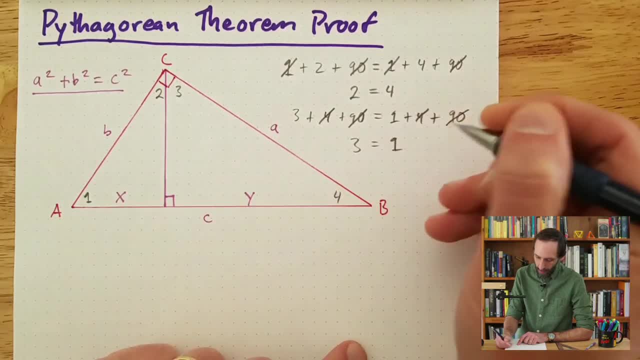 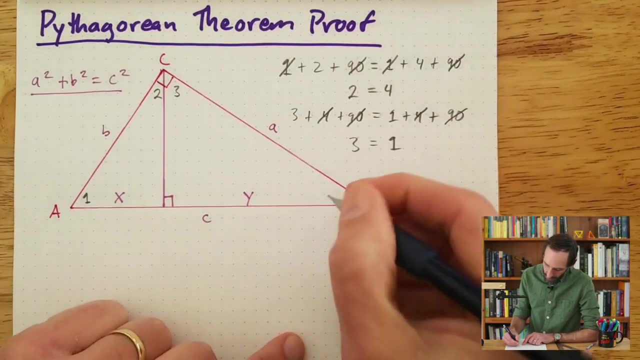 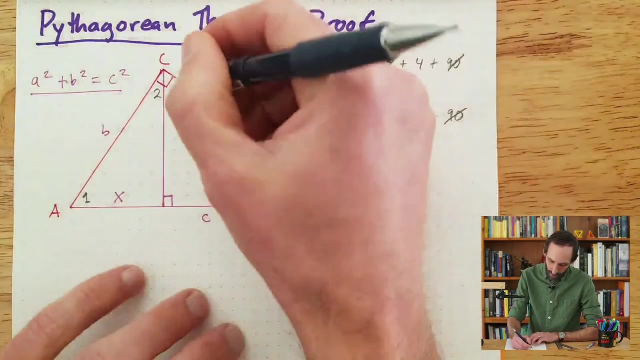 to 1.. So angle 3 and angle 1 are equal. So let's go ahead and erase. let's see, I'll erase this 4, and I'll replace it with a 2.. And then, since 2 is equal to 4, and then, since 3 is equal to 1,, I'll go ahead and erase. 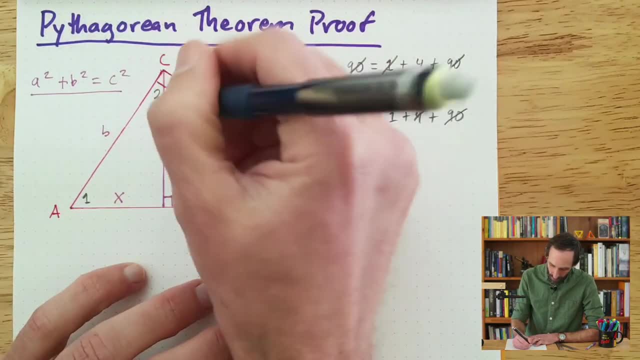 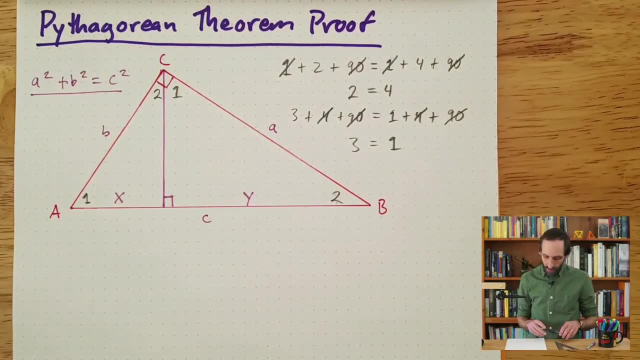 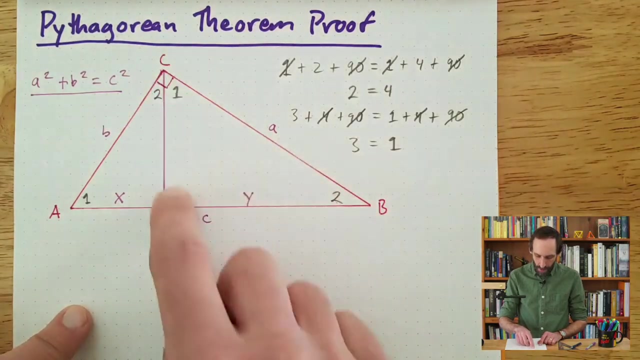 this 3 up here and I'll replace that with a 1.. Okay, now let's look at the three right triangles we see in the diagram. The small right triangle has angles 1,, 2, and 90 degrees. The medium sized right triangle has angles 1,, 2, and 90 degrees, And the big right triangle 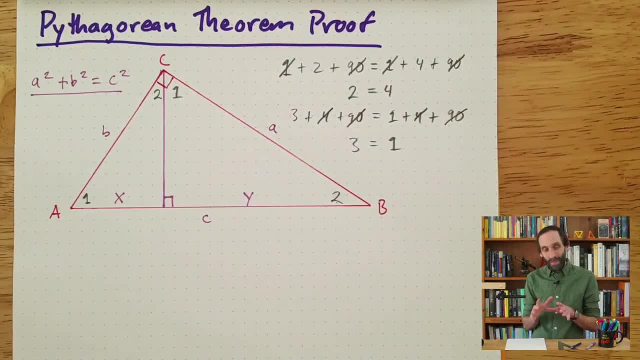 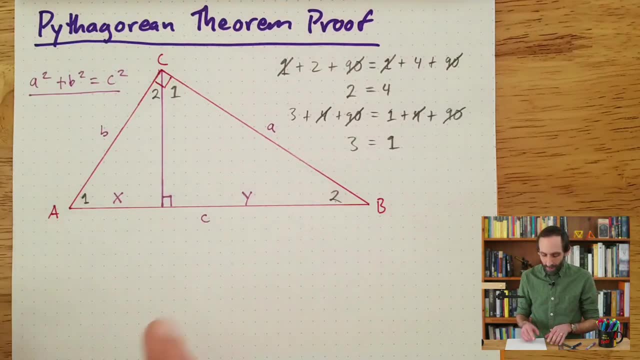 has angles one, two and 90 degrees. That means that this small triangle is similar to the medium triangle, is similar to the big triangle, because all three of them have corresponding angles, equal. That's how we know that they are similar. 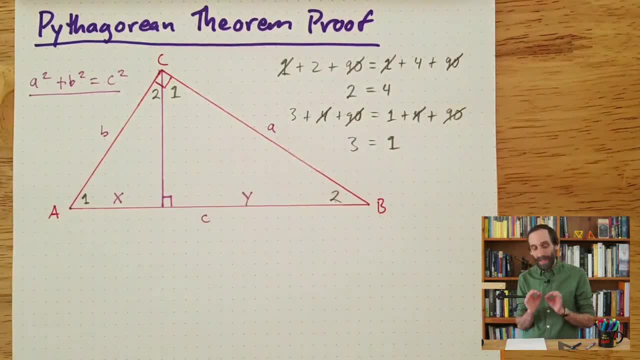 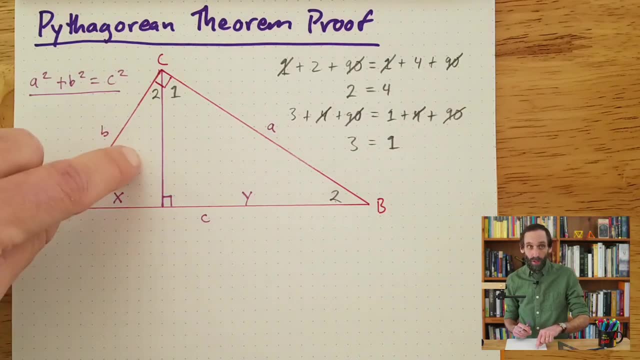 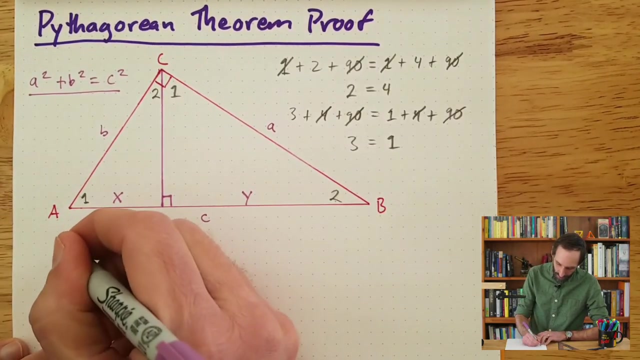 Now we can use the fact that these triangles are similar to set up some proportions. Okay, so first I'm gonna set up a proportion between the small triangle and the big triangle, So in the small triangle I'll use the shortest side, x. 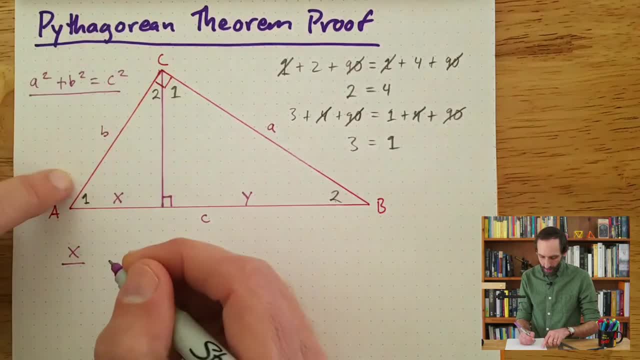 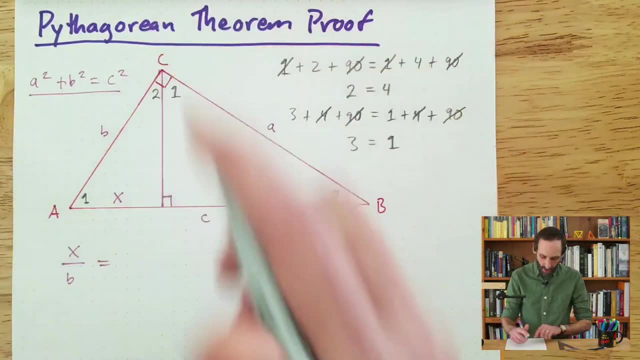 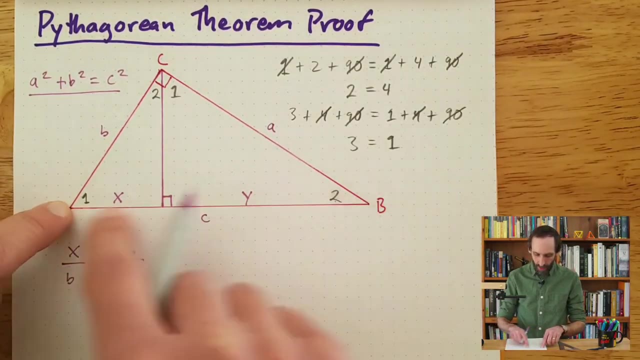 We'll say: okay, x divided by the longest side, b. Well, that must be equal to the shortest side in the big triangle, which is b divided by the longest side in the big triangle, which is- I could say, x plus y, but it's also c. 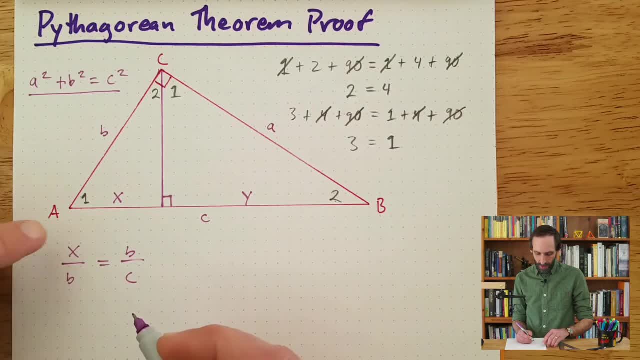 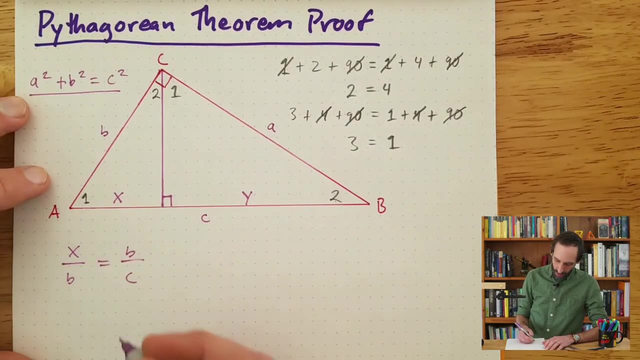 so I'll use that. So x plus sorry, x over b. this over this is equal to this over this, That's using the fact that corresponding sides of similar triangles are proportional. Now let's cross multiply. And if I cross multiply, I'm gonna get b squared. 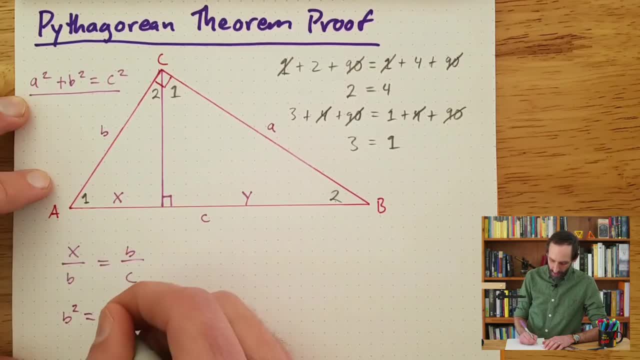 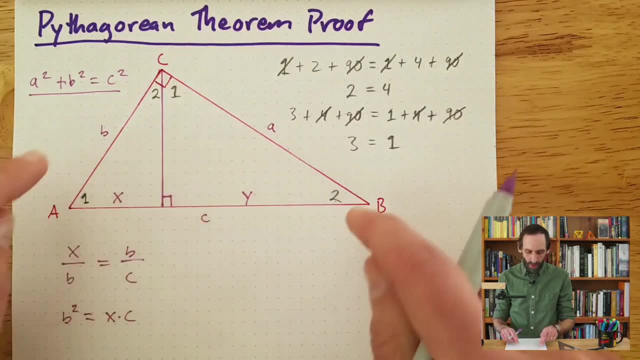 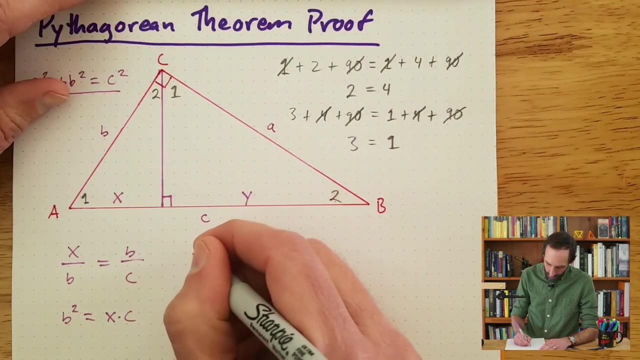 b times b is equal to x times c. Now let's set up a similar proportion with the medium triangle and the big triangle. Now, in this triangle, I'll go with this longer leg y And I'll say, okay, y over the longest side. 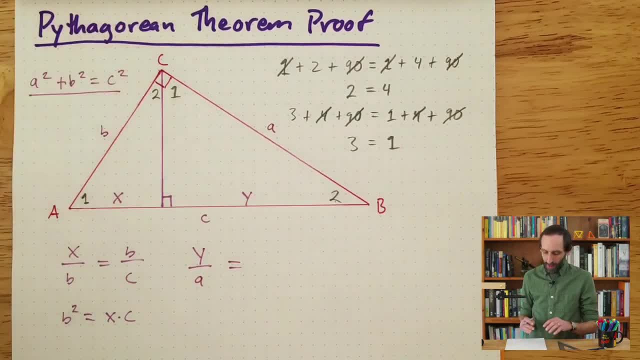 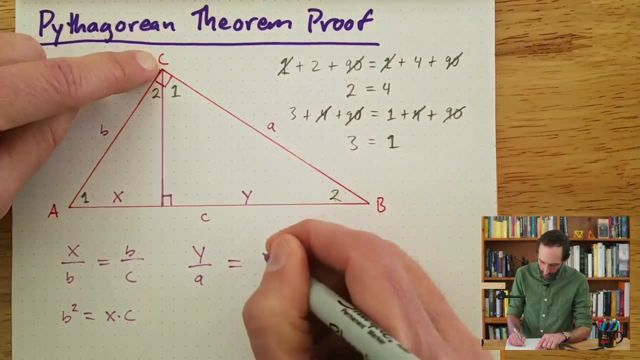 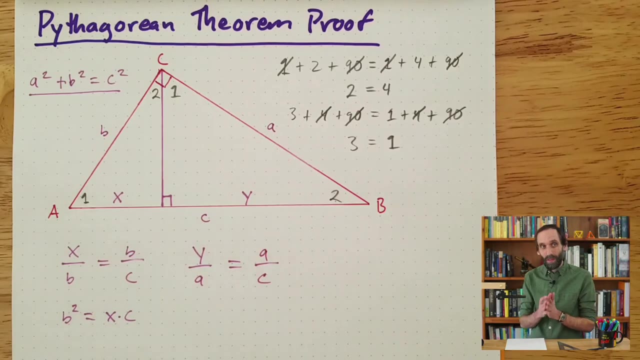 the hypotenuse a in the medium triangle is equal to. that proportion is equal to: let's see this longer leg, which is a, divided by the hypotenuse which is c. Again, using this fact of proportionality, 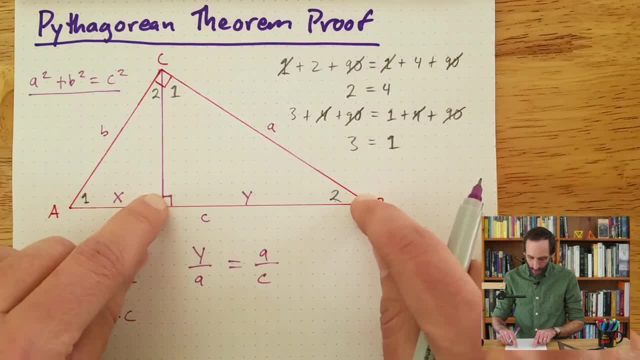 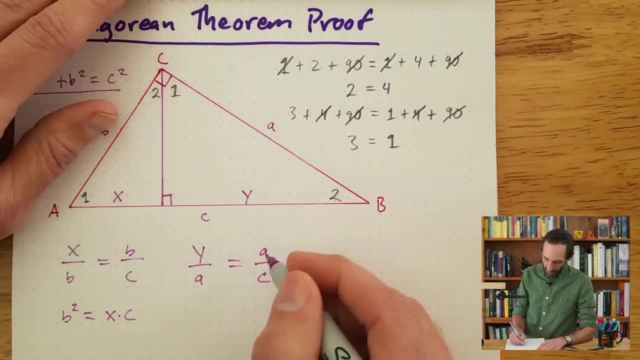 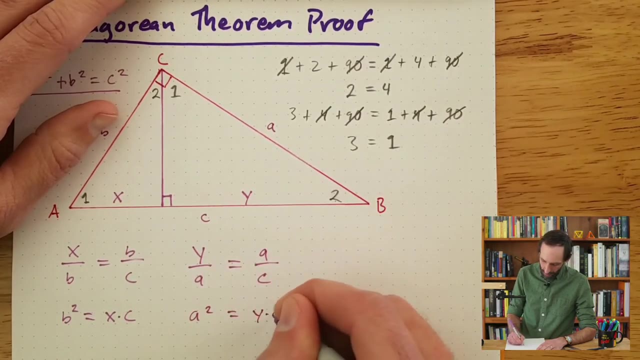 So again, in the medium triangle we have y over a is equal to, in the big triangle, a over c. Once again I'll cross multiply. I'll say a times a, which is a squared, is equal to y times c. 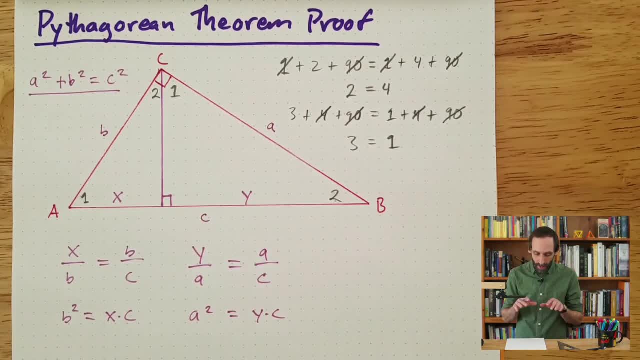 Now, if we look at these two equations, we might realize that maybe we're making some progress, Because here I have a b squared and here I have an a squared, And I want to prove that a squared equals b squared. a squared plus b squared equals c squared. 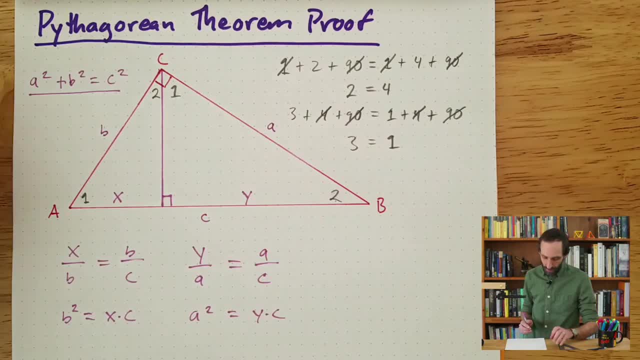 So I'm gonna have to do a little algebra, but I'm getting close. Now what I can do is I can add b squared to both sides of this equation. So I'll add b squared plus b squared You can add. this is something you can do in algebra. 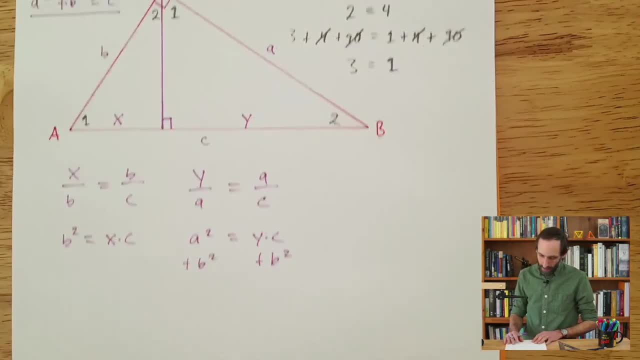 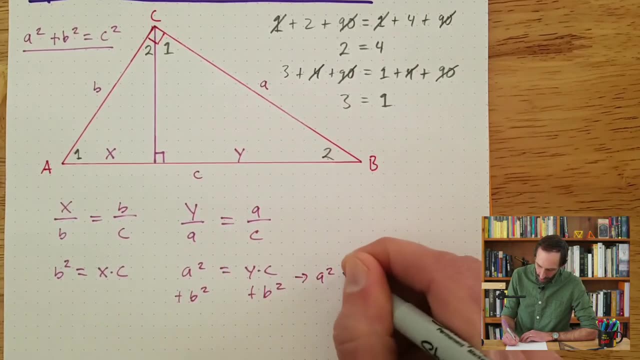 You can add the same thing to both sides of an equation And actually I'll send this over to the right here. So what does that give me? It gives me a squared plus b squared is equal to y times c plus b squared. 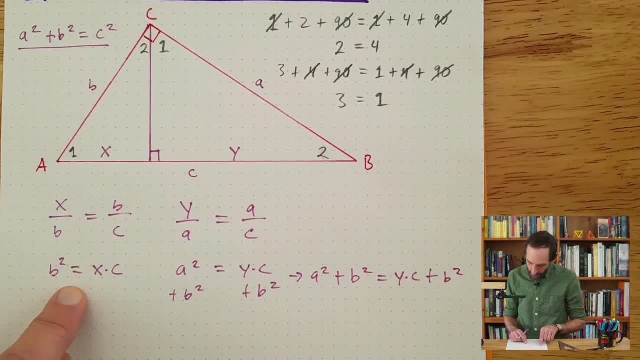 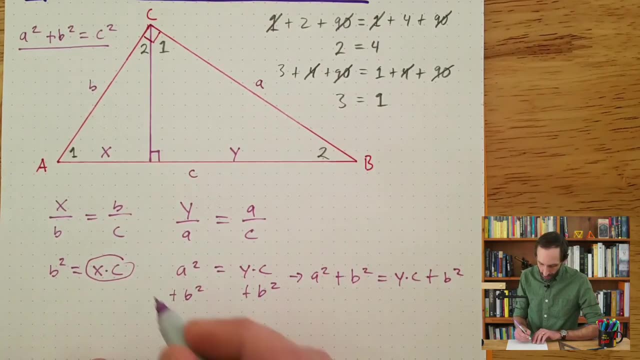 Well, if I look at this equation, I can say: hang on a second, I got this b squared here. b squared is equal to x times c, So let's take x times c and let's substitute it in for b squared. 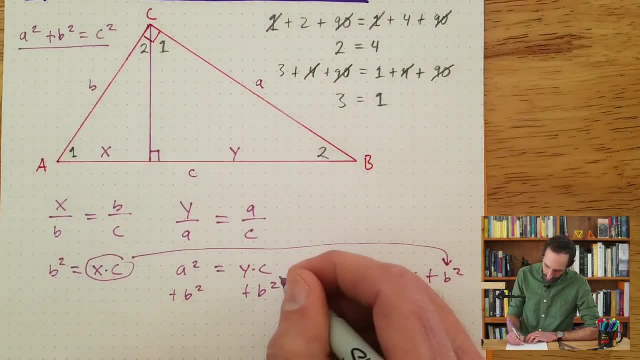 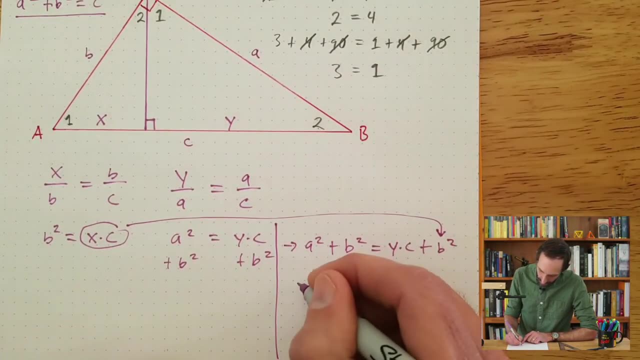 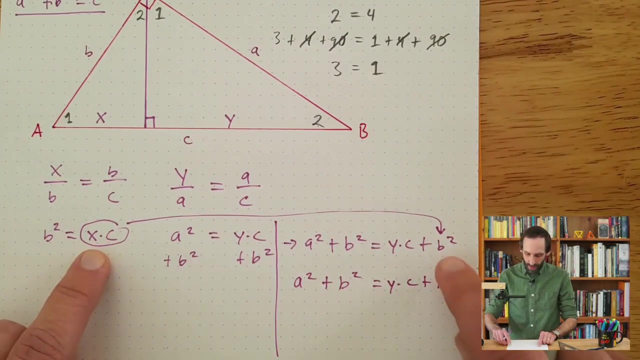 Well, if I do that- and let me just draw a little line here so you can see that these calculations are isolated over here now- I'm going to get a squared plus b squared is equal to y times c plus x times c, because I've substituted x times c in for b. 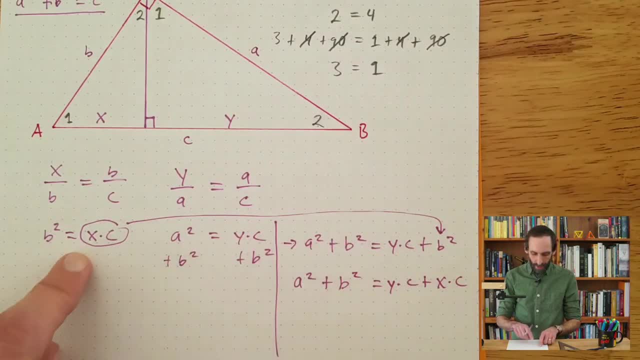 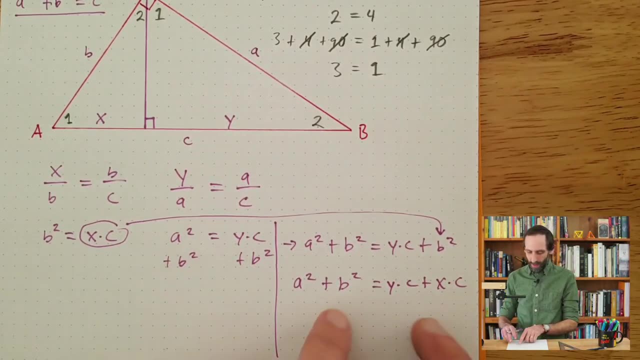 You could also- I mean, you could just say I'll add these two equations and you would jump right to this. I feel like sometimes students might be like wait a second, what allows you to do that? So I thought I'd do it this way, just to make it absolutely clear that you know we're following. 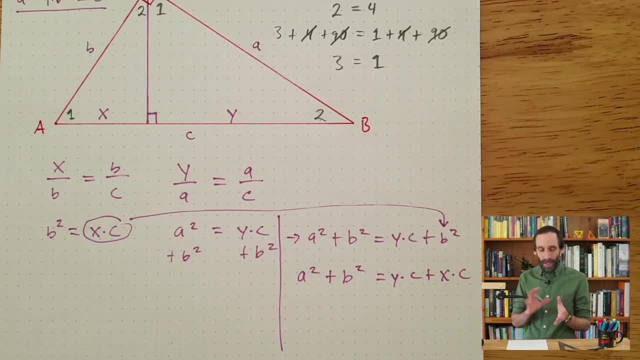 the rules of algebra here right, And it's not too hard to prove that adding two equations together is legal to do in algebra. So yeah, you might even give that a shot on your own time. So now let's think about what. 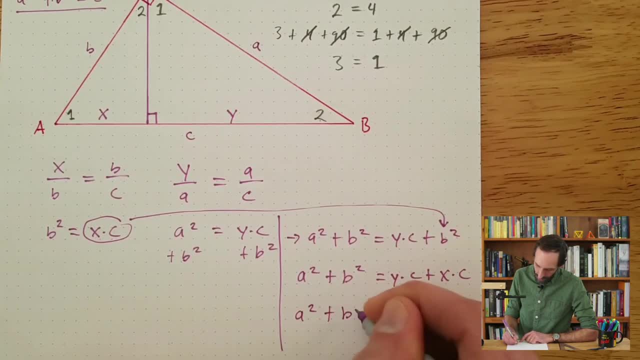 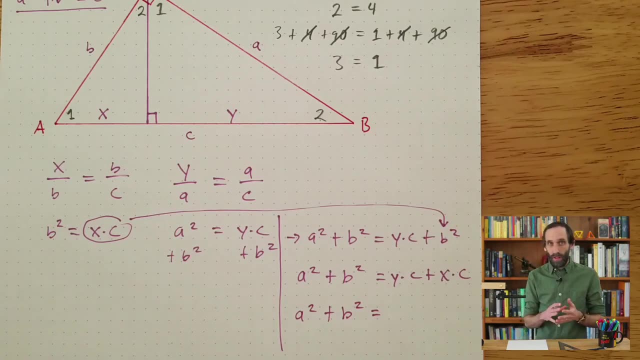 can we do next? So a squared plus b squared? Well, you may recall the distributive property from algebra, which the sort of the inverse of distributing is factoring, And so I can factor a, c out of both of these terms. So let's go ahead and do that. So then I'm going to have y plus x. 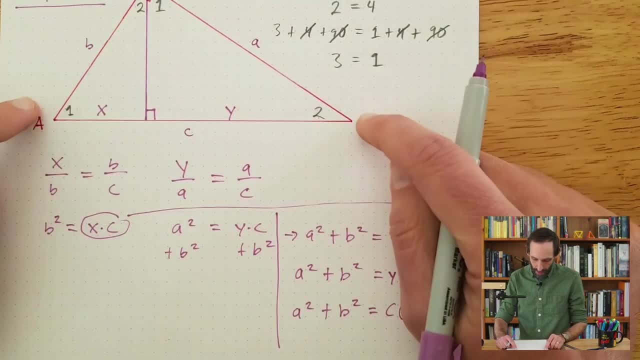 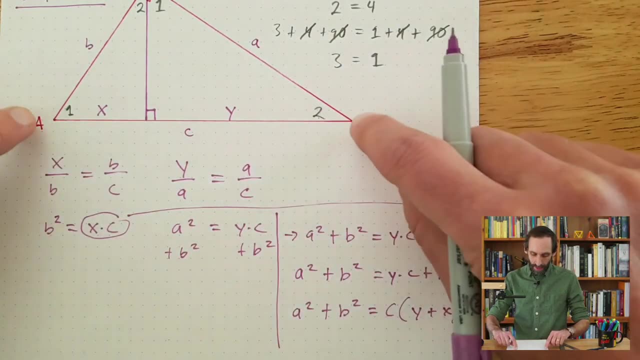 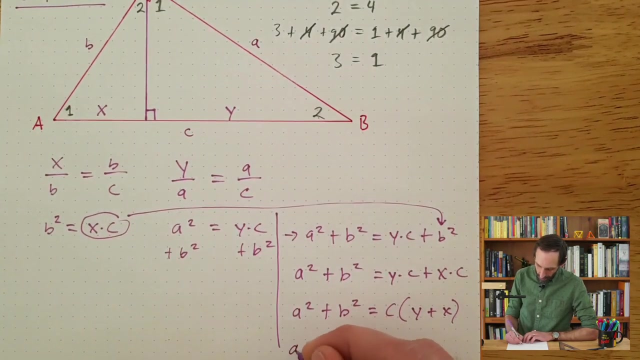 inside the parentheses. Well, let's go back and look at the diagram And we see x plus y. the sum of these two lengths is equal to c. it is c, And so I'll replace this y plus x with c, So I get a squared plus b squared equals c times. well, c, because that's what y plus